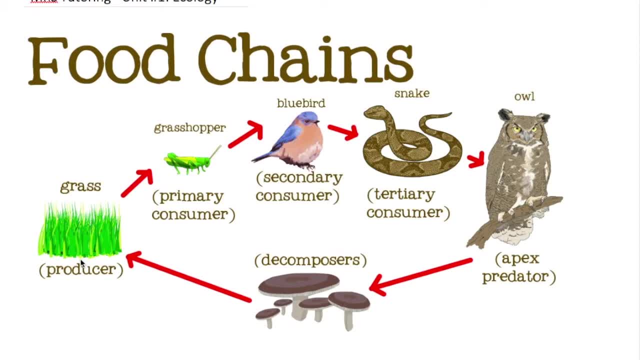 or energy up the food chain. So now let's move on to the second part of the food chain, which are the primary consumers. Well, the primary consumers are basically smaller consumers. They're usually insects or small rodents and usually other animals that rely on the producers for food. 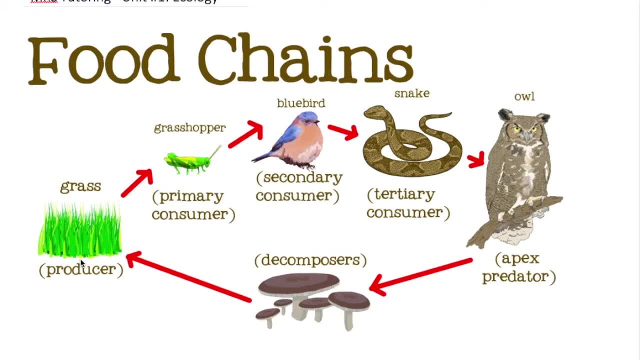 They eat plants and mostly all primary consumers or herbivores. In this case you'll notice that the primary consumer is the grasshopper. Has I mentioned before, the grasshopper will usually rely on the producers for food and shelter. So the producers are given the grasshopper two ways If they many alot of. 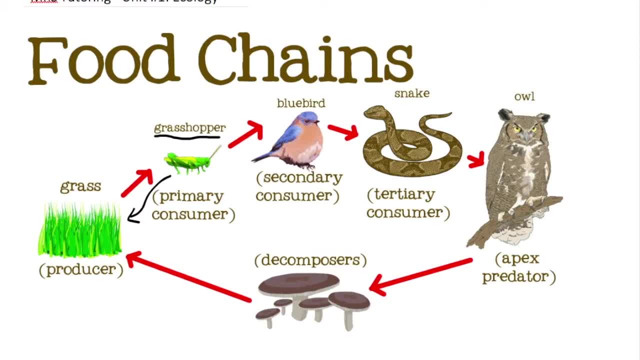 times. if the produce is food generally, they'll take the space between the grasshopper and the pasture for nutrition two-way niche in the food chain. the niche is a role in organism plays in the ecosystem. so in this case the grass is giving the grasshopper shelter. so I'll 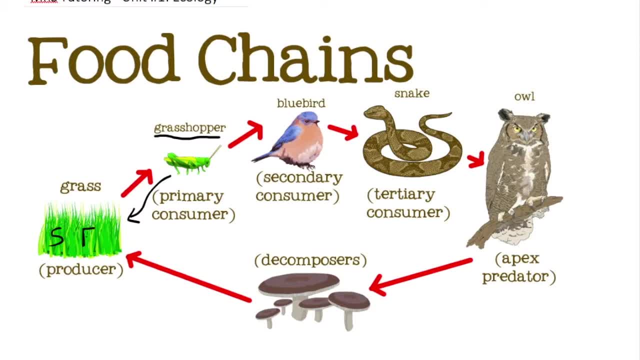 put an S over here and it's giving it food right. apart from that, all the arrows in the food chain go to where the energy goes. so all the, all the grass that's been eaten by the grasshopper gives the grasshopper energy. you do the different. 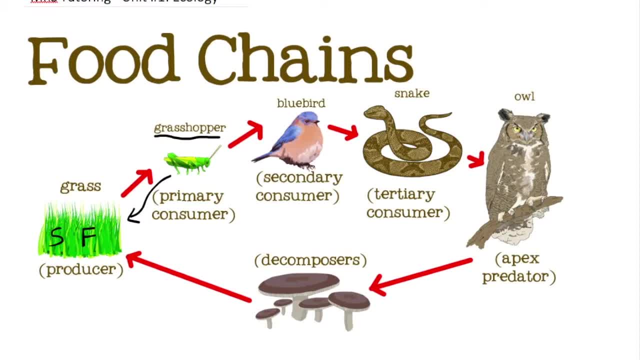 glucose, carbons and everything, every other nutrients in the grass that actually give the grasshopper a sustainability to survive. so now, what, what, what? what do the arrows actually mean in the food chain? well, there's actually different types of arrows in the food chain. in this food chain, you 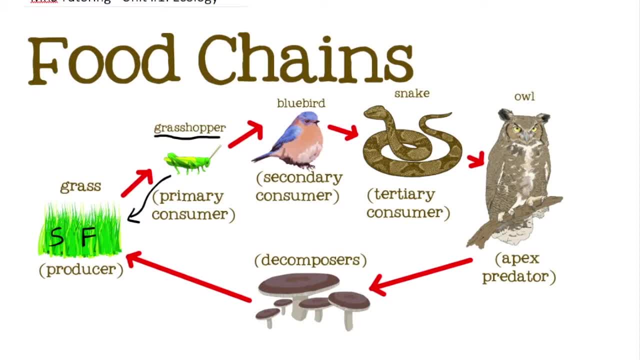 can see that there are only bold red arrows, but usually when there are dotted arrows, something like this maybe, right, it usually means that there is a weak connection between the organism in the food chain. right, this usually happens when, when an organism doesn't mainly rely on such-and-such thing for food, and it also 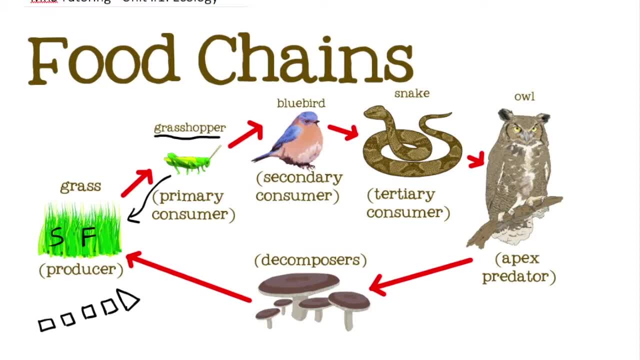 gets its foods or something else which can really cause a weak connection in the food chain. but a weak connection in the food chain is perfectly fine because if, if, if a grasshopper, say, for example, gets its, gets its nutrients, gets its energy from not only grass, but let's say it, 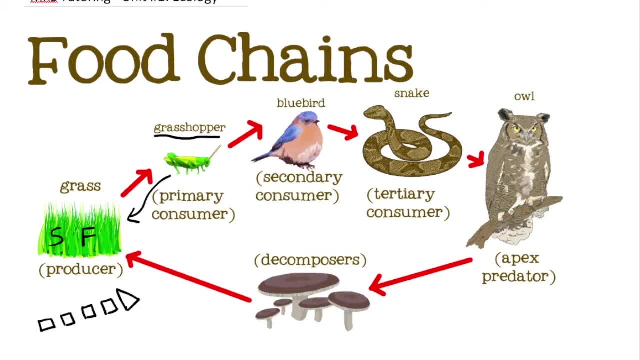 it from. you know, let's say tree bark or something, something other than grass, right, it's a good relation in the food chain because it provides the tree bark or anything else in the food chain with a role to play in the ecosystem. so now let's move on to the secondary consumer and in this case, the secondary consumer. 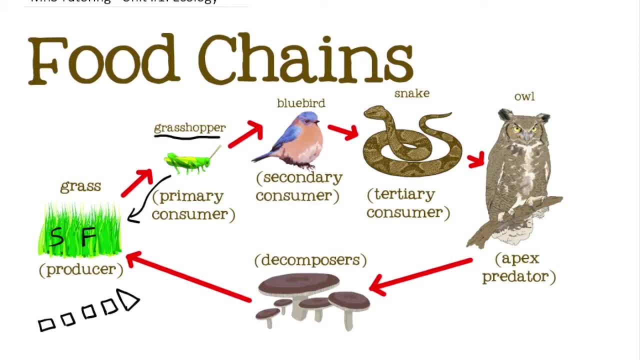 is the bluebird, so the secondary consumers are usually consumers that eat other smaller primary consumers, and usually in this case the bluebird is an omnivore. as they eat some plants as well, it leads ILL eat some plants and berries as well. in a very rare case scenario, the secondary consumer can be carnet. 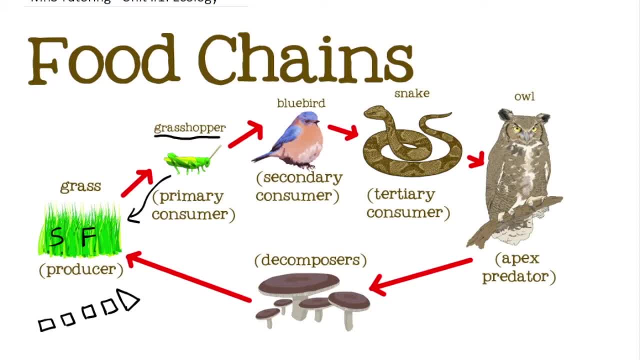 carnivorous, but in this case the bluebird is not. so beside the bluebird I'll just write: it can be either an omnivore- omnivore- sorry, omnivoreuge, you don't want to use phone number, you can definitely use phone number- carnivore- or it can be a carnivore right now. let's move on to the tertiary consumer. 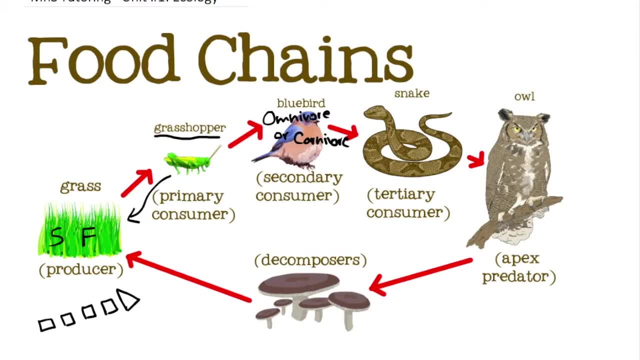 um the tertiary consumer is usually um the consumer that's on the top of the food chain and um. this usually means that the tertiary consumer relies on everything below it in the food chain, which in this case is grass, the producer, the grasshopper, um the grasshopper. 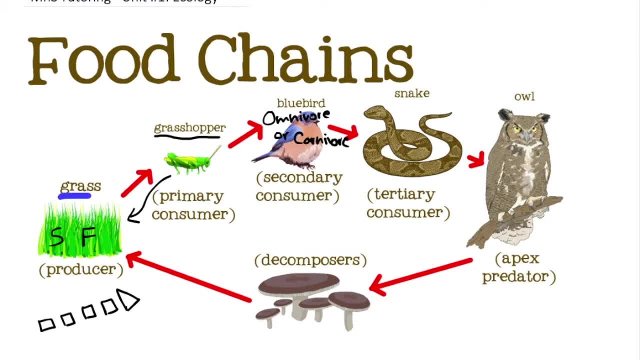 and the bluebird for food, and, um, the the snake does not really have any specific eating habits and in this case it it shows us something really about a lot of the tertiary consumers. tertiary consumers, um, since they're so high up on the food chain, um, they can really eat anything that they. 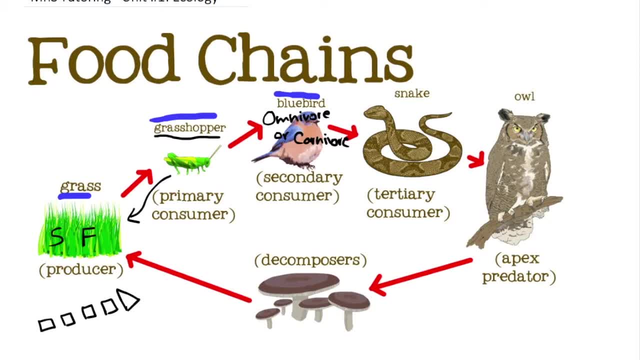 want. so usually- uh, usually, the snakes will eat anything that they can get their hands onto and um, being the tertiary consumer, um it, the snake, has a really big job to play, as he really manages everything below him in the food chain. um, and the tertiary consumer, um, usually, 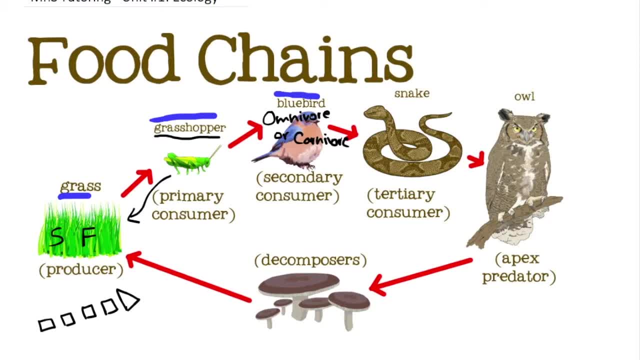 always eats primary, um or secondary consumers and um, sometimes even producers, um, say, for example, a. a bear, um, let's say a grizzly bear, is sometimes considered, uh, a tertiary consumer, depending on the ecosystem, and it is an omnivore as it sometimes eats um a lot of producers as well, like some, something like. 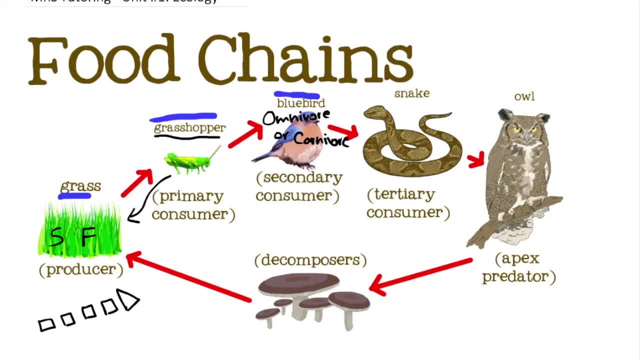 fruits, berries, um some grass, shrubs and so on. so now let's move on to the last actual living um living, uh, um, sorry, living uh- organism in um the food chain, which is the owl. the owl is the apex predator, as it has nothing it can- um, really it can. there's nothing it can be eaten by, and it's on top of everything in the food chain. 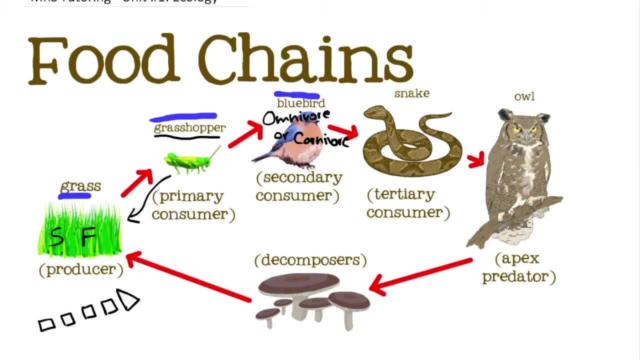 well, some of you may be thinking. well, i thought you just said that the tertiary consumer was on top of the food chain. well, it's really not, because the tertiary consumer, um, just gives its energy to the owl. the tertiary consumer has a really big role as to controlling the food chain, but something 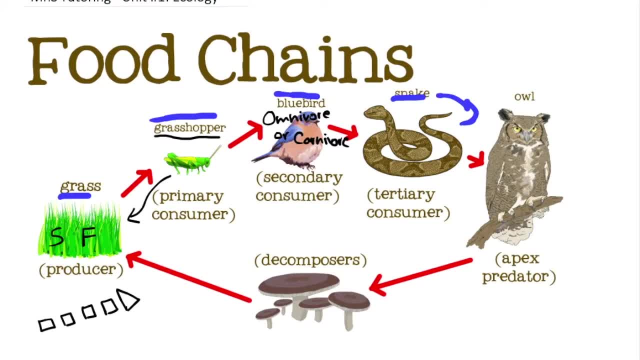 something even bigger than that. an apex predator is not present in all food chains, but in a food chain there is a lot of a different variety of species and organisms. um an apex predator is sometimes needed to control all the organisms within it. so in this case, um the apex predator. 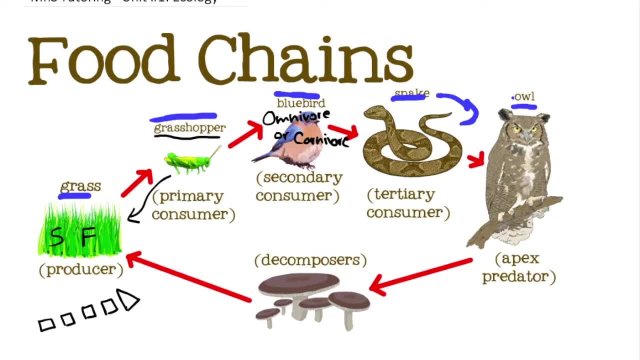 is the owl and, as you may notice, the owl may eat anything from um snakes to other smaller rodents that can be considered uh primary consumers. so, again, the owl is on top of the food chain and after the owl dies, um, or it naturally um, you know uh. 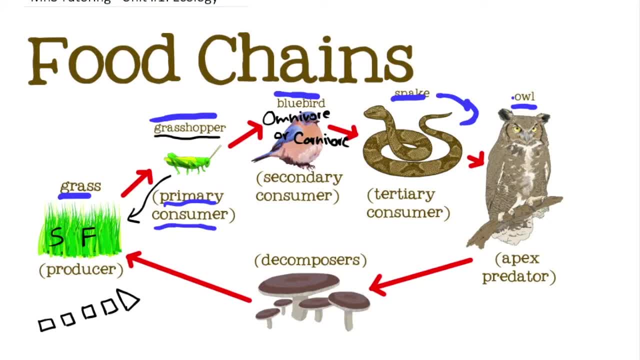 expires um, the owl then gives its energy to the decomposers. the decomposers are a very special, very special organism in the food chain because they not only rely on the food of dead and um dead and decayed animals, but they really bring the energy um to a cycle in the food chain and 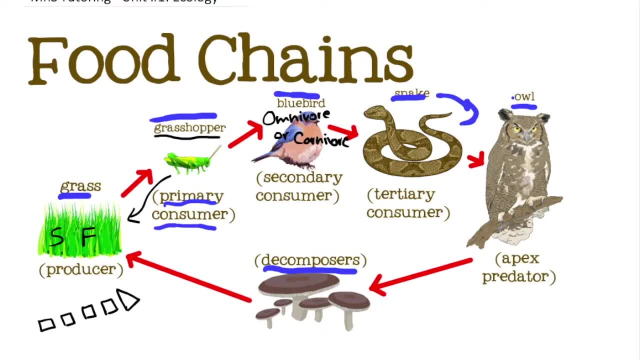 without the decomposers, all the energy would just die off um as the apex predator. so without the decomposers, this arrow would never be there. so the owl is on top of the food chain and it's there because there's nothing to transfer the energy from the owl to back to the producers. so 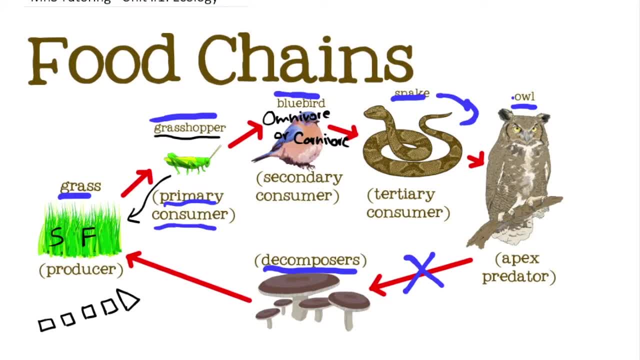 the decomposers play a really big role in the ecosystem, as they keep the energy moving back to the producers so as to where it came from, using photosynthesis, of course. so what decomposers actually do is, um, they decompose as the name suggests and as the owl dies, they decompose a. 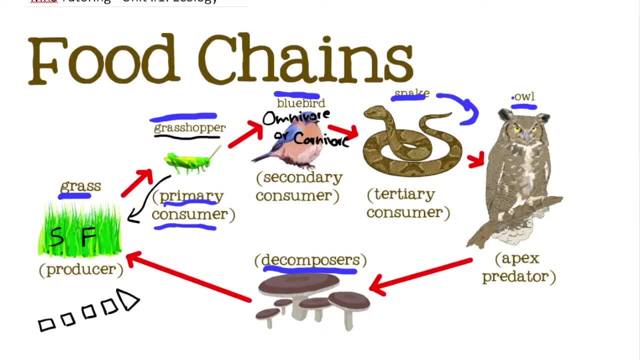 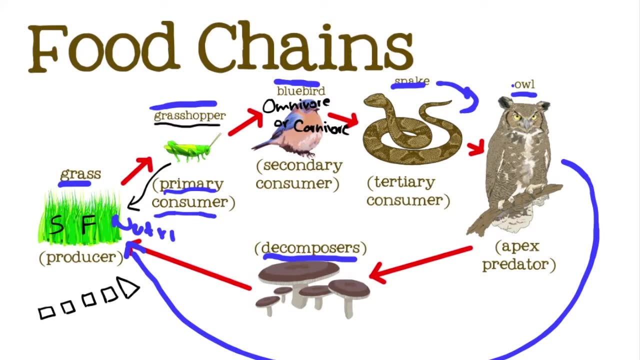 lot of the owl's nutrients in back into the soil. and what this does it? it provides the grass with a lot of nutrients. so basically, all the nutrients from this owl then go to the grass. right, it provides it with many nutrients, right and again that that's why decomposers are one of. 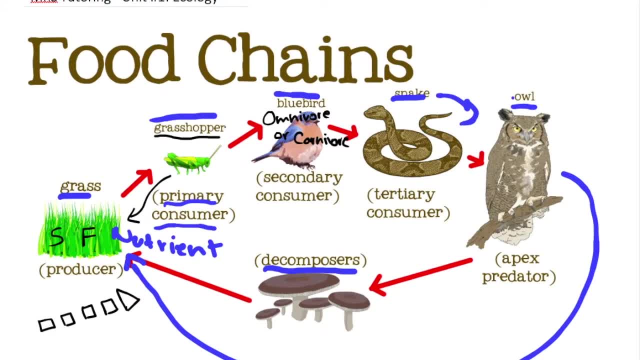 the most important parts of the food chain? um. there's in this food chain, um there's not really any scavengers. the scavengers are any organisms or species in the food chain um that rely on other dead animals for food, but they they don't really help. 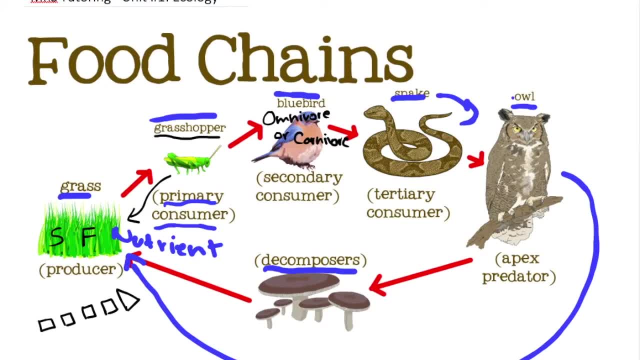 producers. they rely on the food for themselves, so the scavengers would really be something outside the food chain and they would just rely on basically any dead food that they could get their hands on right, not really looking at what it is or, um, and really in a role they would play. 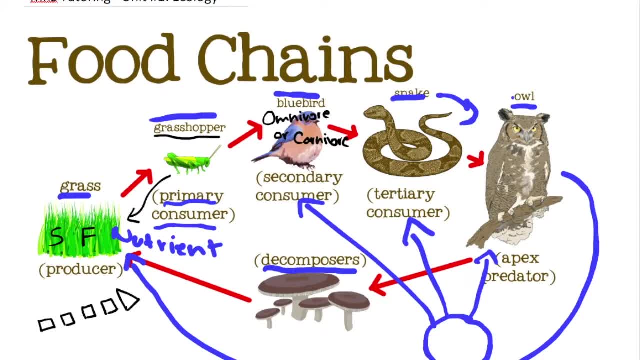 in the ecosystem. right, they just manage all the decayed dead waste, preventing a lot of the diseases in the ecosystem itself. so now let's move on to invasive species. well, what are invasive species? well, invasive species are species that are not native to an ecosystem, and what happens when um there's an invasive species in an ecosystem is the entire. 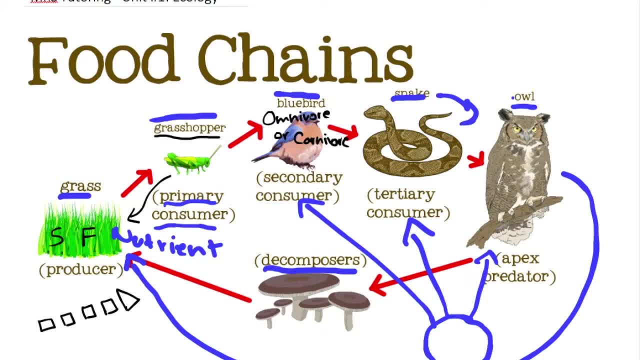 food chain collapses. well, how is this the case? well, recently, um i know, in ontario, the asian longhorn beetle was shipped um, accidentally, of course, from china to canada, and it's been destroying many of the ecosystems the years to be thriving ecosystems that have been going on for years and years in canada. 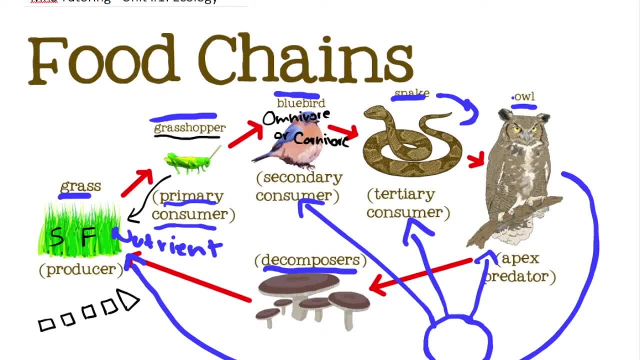 and what invasive species do is they don't really belong in the food chain, uh, but they take a lot of the resources. so say, for example, i have the asian longhorn beetle over here and it's in the middle of the food chain. right, the asian longhorn beetle, since it does not really. 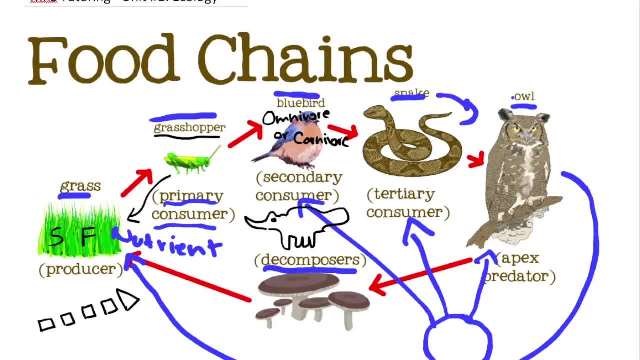 belong in the food chain. there's nothing, um, that's not going to be able to survive in the food chain. there's nothing that that can get its energy. there's nothing that is adapted to actually kill it as prey and then eat it. so what the asian longhorn beetle does is, in this case, it usually 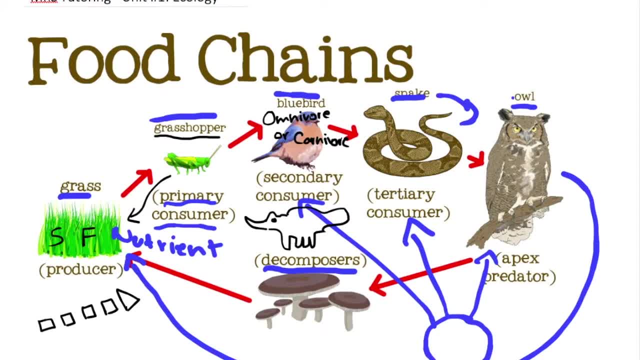 feeds on mostly um grasshoppers and grass as well, so it usually takes the energy from the grasshoppers and the grass right, and since there's nothing to really control the asian longhorn beetle's population, um, it just keeps on overpopulating until, um, there's way too many of. 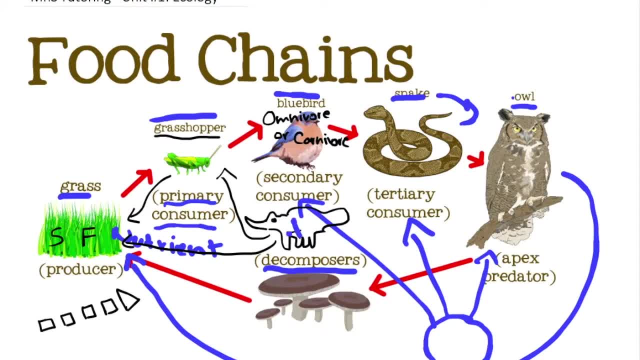 the asian longhorn beetles. so continuous overpopulation of the asian longhorn beetle and then, after this happens, um. such a large population of asian longhorn beetles need so many more resources to be able to sustain the population. so slowly you'll begin to notice. 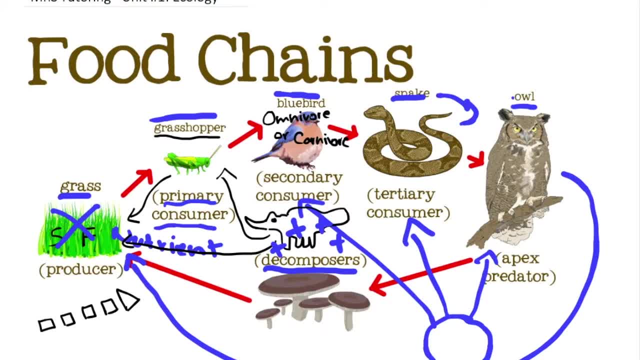 in the ecosystem that there is no more grass, because the asian longhorn beetle usually take all of it, um, as a means of sustaining the population. as there's no more grass, there becomes no more grassland, and there's no more grassland. and there's no more grassland and there's. 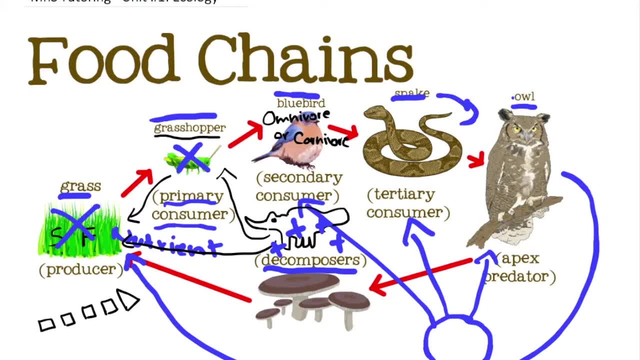 hoppers, because grasshoppers now no longer have a means of getting energy and since there's no grasshoppers, there was really no secondary consumers. there's no bluebirds- sorry, since there's no bluebirds, there's no snakes, because now snakes don't have a means of getting any energy. or 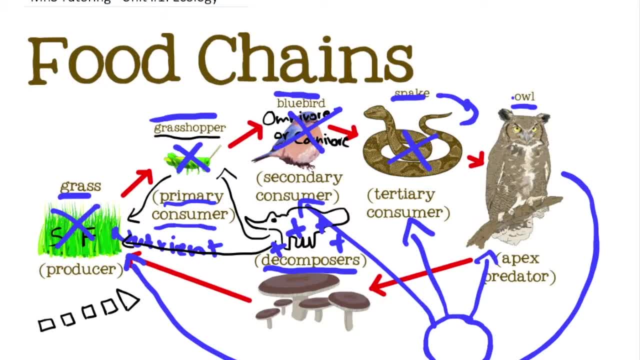 nutrients. and now, since snakes are really extinct and they they are no longer in the ecosystem anymore, owls, the apex predator, everything that's controlling the food chain, now no longer has anything to get its energy from and sooner or later the owl is usually dead or it goes extinct. 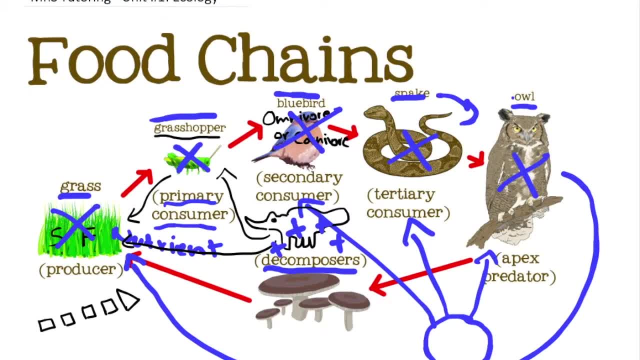 in the specific ecosystem, and now that the owl is gone, the decomposers have nothing to decay into- back to the soil, as there's no other organisms left except, of course, the asian longhorn beetles. and eventually, as the whole ecosystem falls apart, um the asian longhorn beetle as well also expires, um, it also dies off, and the population.